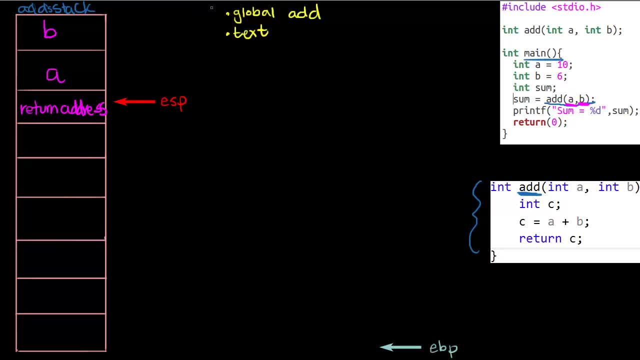 We'll be starting here, So I won't explain these two lines in this, in this tutorial. but, um, hopefully I'll get around to it in another video. So anyway, um, So sorry, You always want to write that before you write the code, and we'll start off. let me put it in a different color. 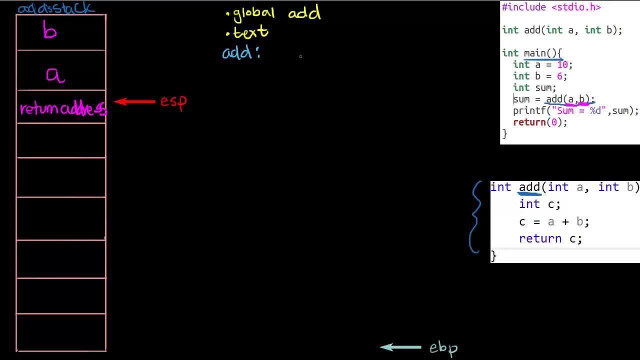 We'll start our code at this add label. So this add label. like I said before, Whenever we're writing a function function in assembly, we always want to start with this thing called the prolog. so the prolog- I explained this in another video- goes something like this: 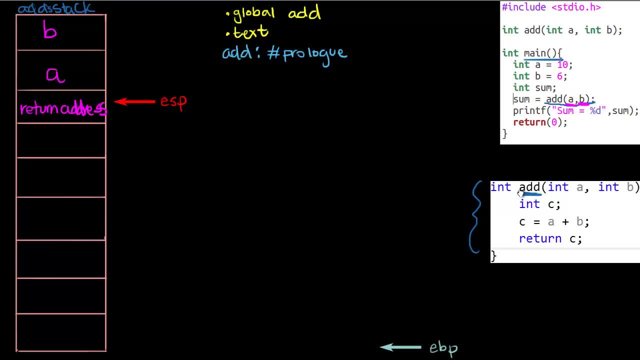 the prolog. let me draw this in different color. prolog goes something like this: push EBP and move ESP to EBP. so let's go at this line by line. so we're saying so when we get to this line here, basically we're saying: all right. 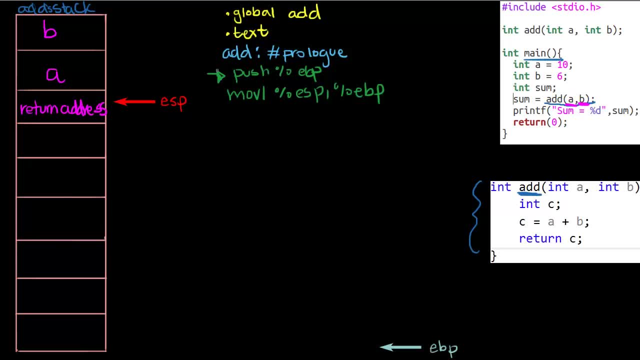 push the value EBP, the value of it, that though, all the value that it had before it, actually before we do anything with it. So I like to call that the value. I like to call that value old EBP. So in our drawing here, we'll push on old EBP. So we're pushing on old EBP and we know that when that happens, our ESP register will be pointing to the top of the stack. 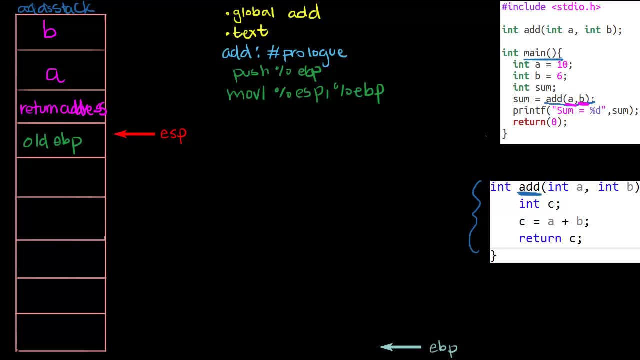 Oh yeah, one thing I didn't really touch on was forgot to say that these are high memory addresses and goes to low memory address. So yeah, so now that we have that, this next line, this next line here, it's basically telling us in simple words, it's telling us: alright, make EBP, make EBP point to whatever ESP is pointing to. 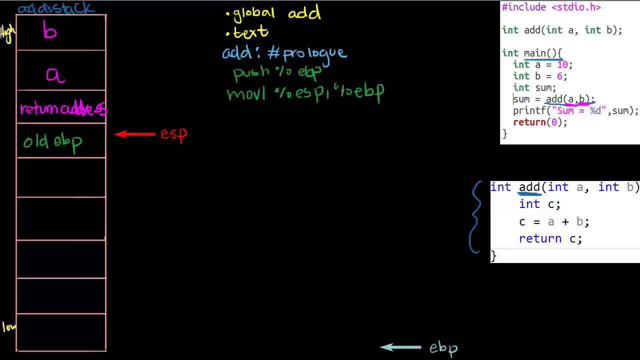 So EBP will basically. so we're basically moving the value, we're copying the value of ESP into EBP and that just means EBP will point to the same thing that ESP is pointing to. So EBP- let me get EBP. EBP will be pointing to. let me move ESP up, EBP will be pointing to. 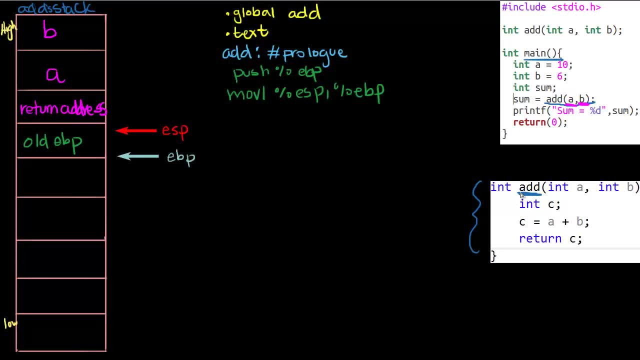 Oh crap, EBP will be pointing to the same thing that ESP is pointing to. Hopefully, you see that now. Alright, so that's the prologue. We always start with that and we'll see in this video why exactly we do that. 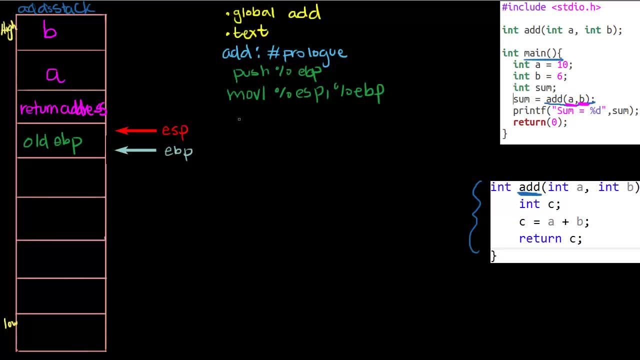 So, anyway, after we do that, like I said in my calling conventions, the GCC calling conventions video, I said that, well, when we're getting called on, since we're going to be the add function, in this case main is calling us. so we're the callees. So what does the GCC calling conventions tell us? 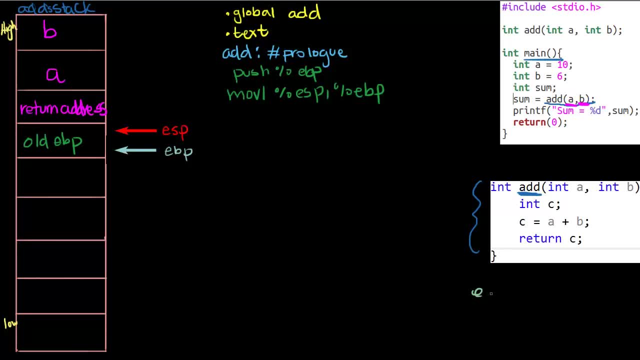 Well, it tells us that the registers EDI, ESI, EBP and EBX, they gotta be when our function terminates, they gotta be the same values that they were when we were called by main. So what I like to do and a lot of people like to do, 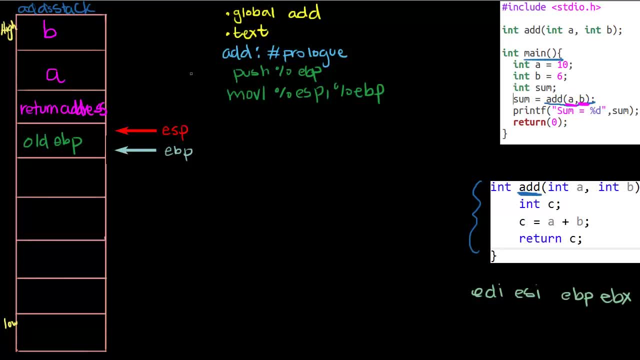 is: we save them onto the stack, No matter what, just save. just as soon as you do the prologue, just push all those registers onto the stack and you can always pop them back off. You always have them there, so it's kind of an insurance. So let's do that. 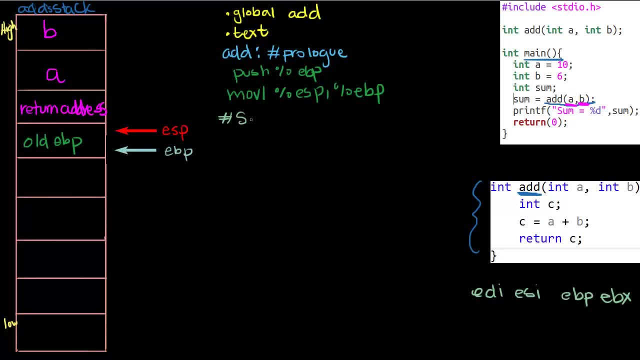 So we'll here, we're basically saving live registers, So we'll save all these live registers. So, registers, we'll push them on, we'll push them on, we'll push. let's push ESI, let's push EDI, let's push. since we already pushed EBP up here in the prologue, we won't have to push it. 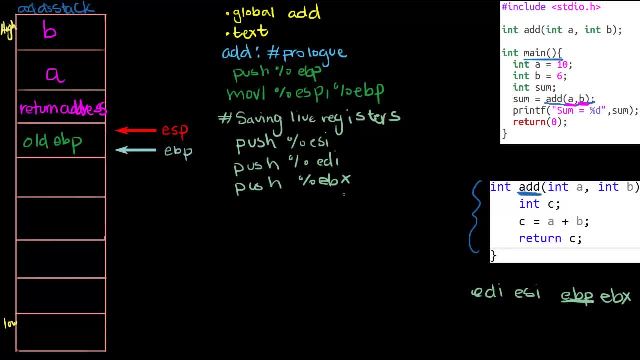 So we'll push EBX last. So yeah, so now we have all of our registers saved and this is how it'll go. it'll it'll, it'll basically push them down here, so we'll have: ESI was the first one that we pushed, EDI was next and finally EBX. we pushed all those things. 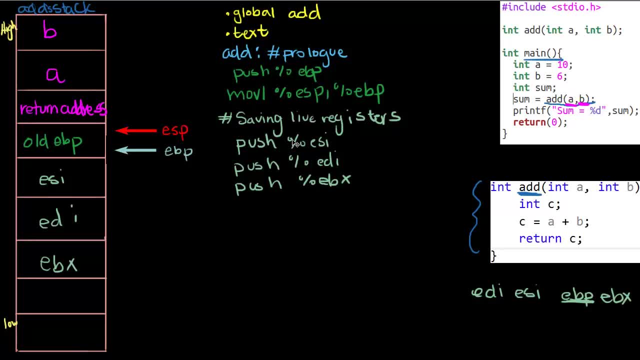 So we know that because of this, ESP, which we said always has to be pointing to the top of the stack, So ESP won't be pointing up here anymore. ESP will actually be pointing to- let me draw this in red- ESP will be down here now. 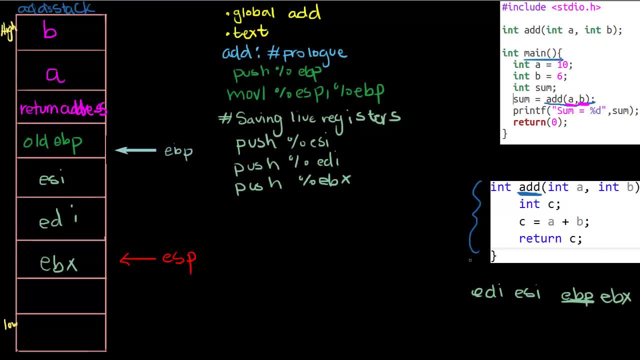 ESP. So ESP moved, alright cool. So we got all our all our live values, live registers saved. We got that insured. so now let's move on to Well, to let's saw. the next thing in our C code is we declare this variable C. so how we 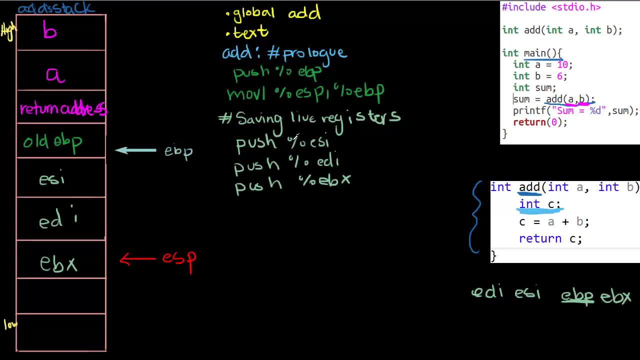 write that in assembly is basically: we're gonna, we're gonna make some room for this variable C, since we really haven't declared anything in it, so we really haven't made it any value. we'll just- this is how we do it. well, we're gonna, let's see, make room for C, which is basically declaring it, so we'll make. 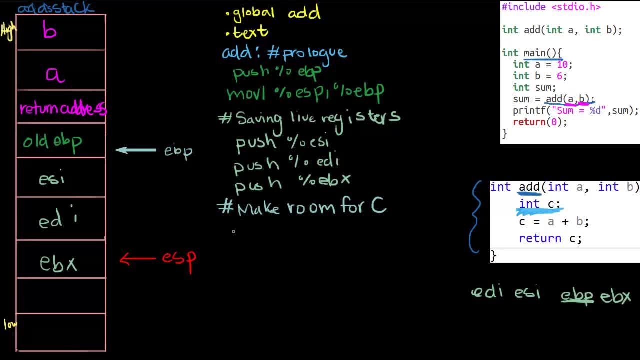 some room on the stack for C. so we're gonna. so how we do this is we're gonna move ESP down and it's just gonna, it's gonna make some room for for C. so, basically, by moving ESP down, let me draw it. so, by moving ESP down, 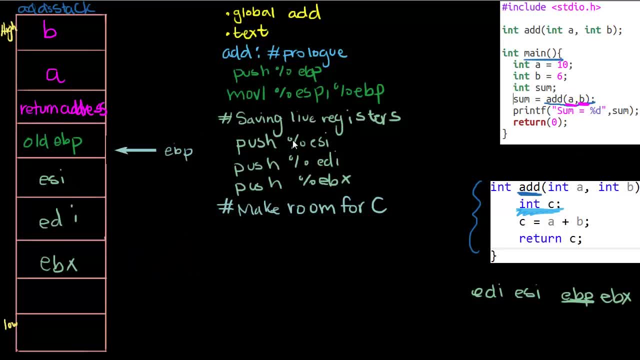 by moving ESP down. it'll be moved down here, ESP, and we know that this is just gonna be blank for now. but we'll just say, okay, this is gonna be where C is gonna lie, so C is gonna be right here, all right. so that's basically this line.